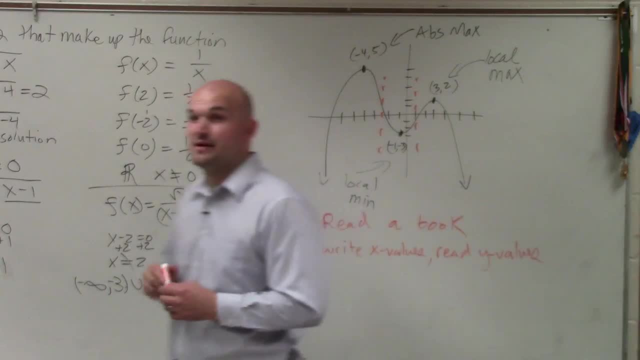 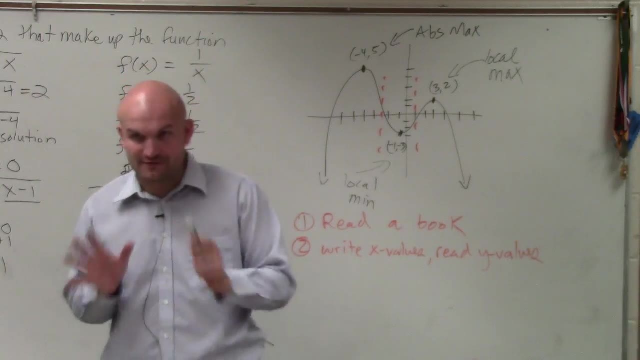 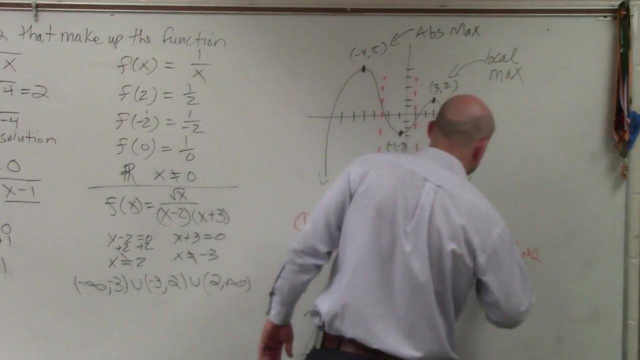 So the thing that comes confusing with this is number one. the notation looks like domain and range, But I want you guys to understand this is a different type of representation that we're doing. So, first of all, read a book. Why am I talking about reading a book? Because I want you guys to read this book from left to right, Because basically, what we're doing is we're going to tell a story. 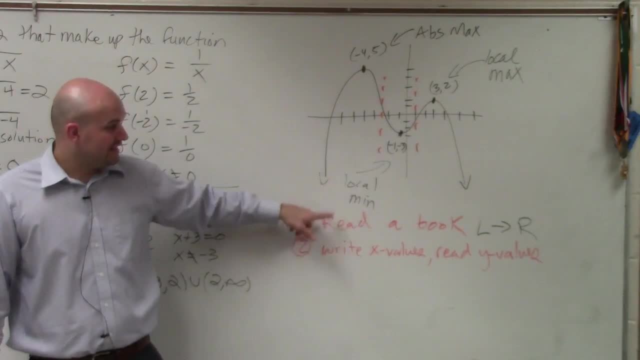 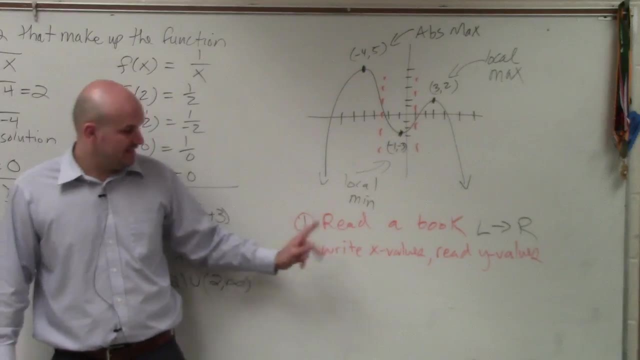 We're going to tell a story of what this graph is doing. It's either increasing, decreasing or constant. Now the other thing is how we're going to tell our story is we're going to write down the x values, and then, of the x values, what are the y values doing? 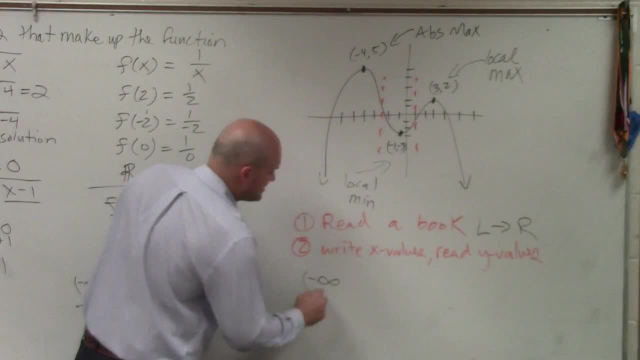 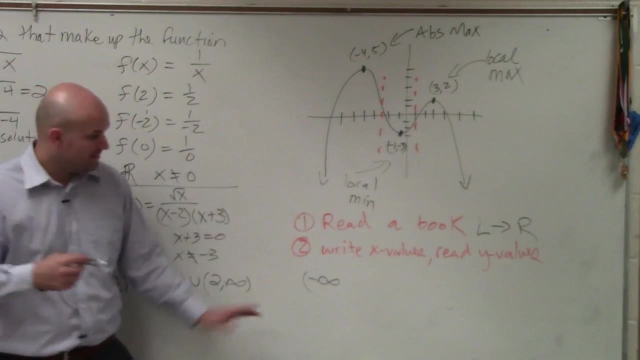 So what we're going to do is we're going to start from negative infinity. It's like the start of time. So, as we're going from negative infinity, which is actually negative infinity down here, but x value, Remember what we're talking about- We're writing the x values. 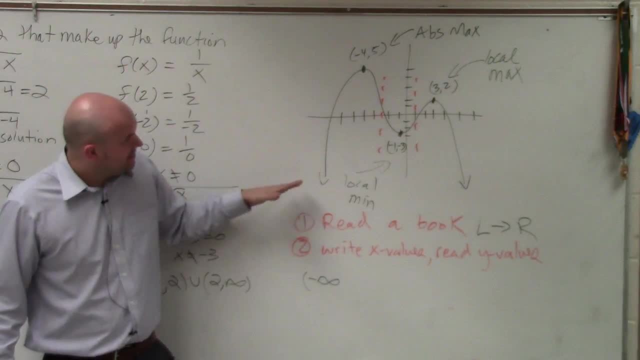 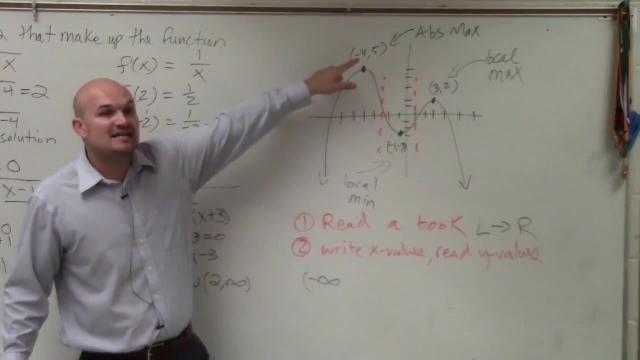 So when the x value is negative infinity and I'm creeping up, then I shoot up all the way up here And then I hit this apex, right The top of there. So from negative infinity to the x value of negative 4, what was the graph doing? Increasing, decreasing. 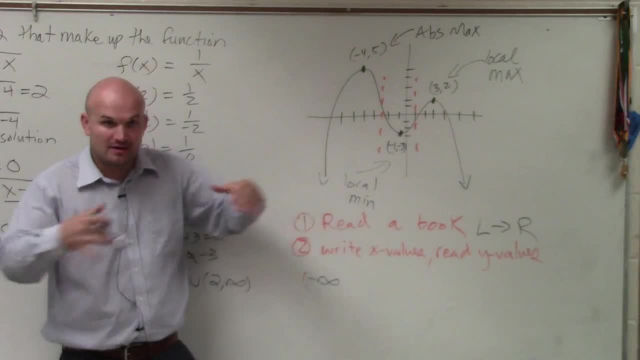 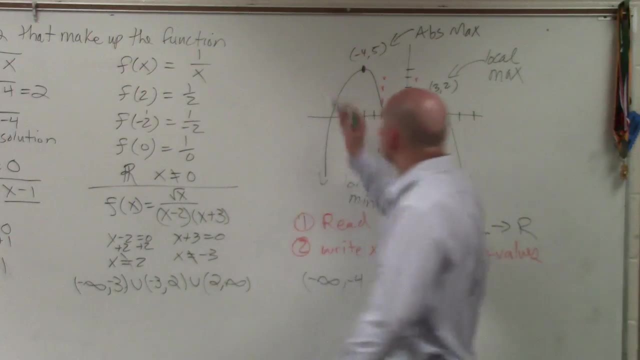 Increasing Right. The y values were increasing right, From negative infinity, from the x value- negative infinity- to negative 4, the graph was increasing. So you'd write negative 4.. Now is negative 4 a part of this graph? Yes, So it's a parenthesis. It's included, right. 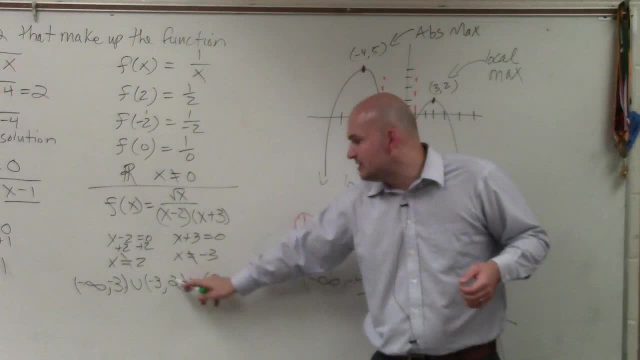 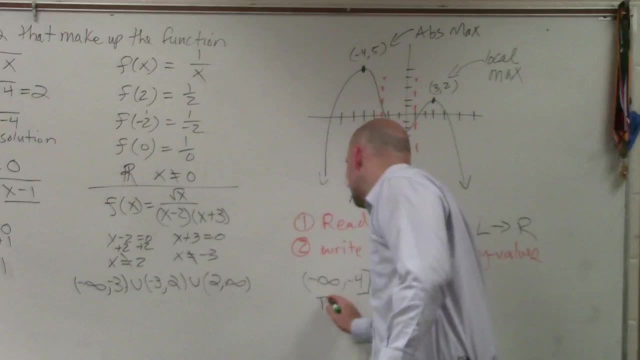 I didn't do that for domain and range over here, Because 2 and negative 3 aren't included. Those are undefined, So we use parenthesis Then, so it's increasing. This is not domain and range, though, so I'm not going to union them, I'm just going to put a comma. 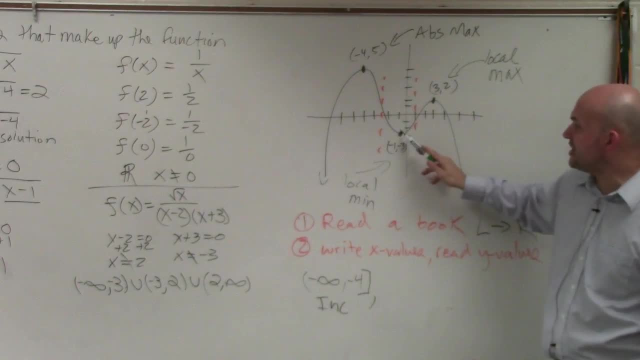 Then from the x value negative 4, to the x value negative 1,. the y values are doing what? Decreasing? So you'd write from negative 1,- oops, I'm sorry- from negative 4 to negative 1, the graph is decreasing. 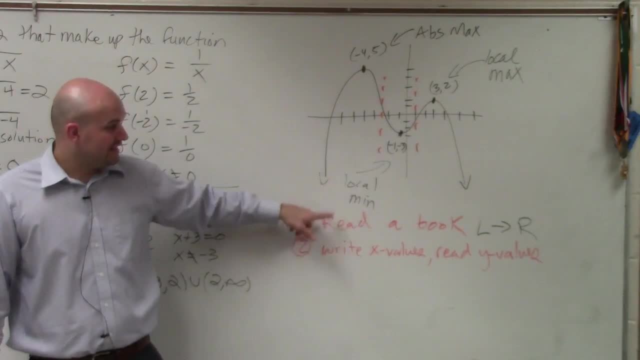 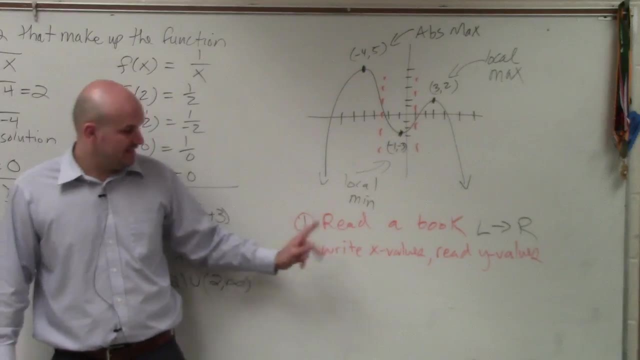 We're going to tell a story of what this graph is doing. It's either increasing, decreasing or constant. Now the other thing is how we're going to tell our story is we're going to write down the x values, and then, of the x values, what are the y values doing? 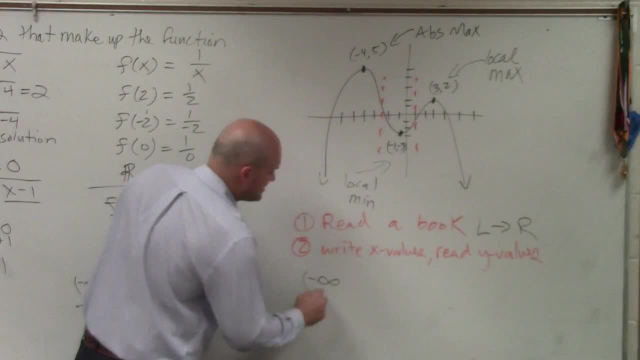 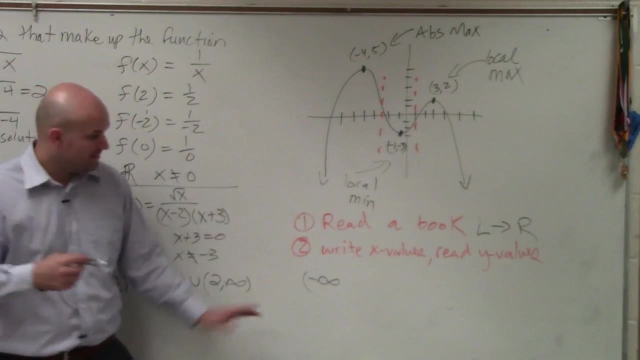 So what we're going to do is we're going to start from negative infinity. It's like the start of time. So, as we're going from negative infinity, which is actually negative infinity down here, but x value, Remember what we're talking about- We're writing the x values. 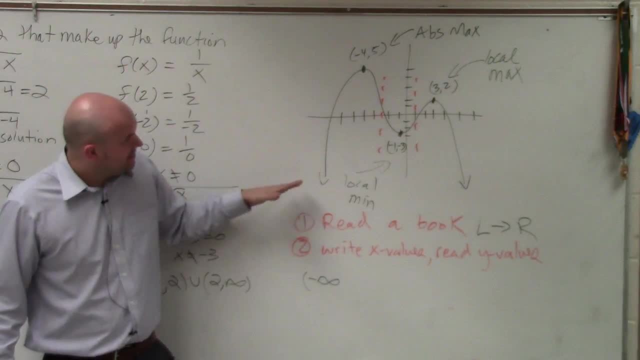 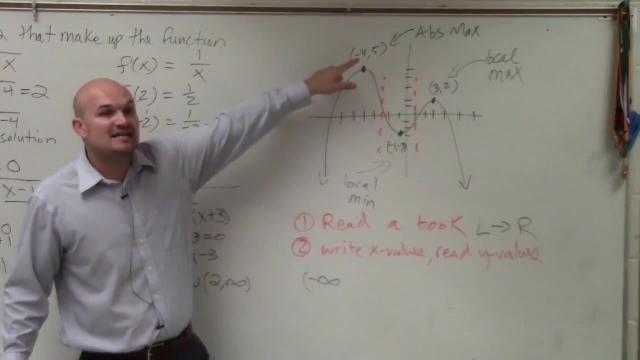 So when the x value is negative infinity and I'm creeping up, then I shoot up all the way up here And then I hit this apex, right The top of there. So from negative infinity to the x value of negative 4, what was the graph doing? Increasing, decreasing. 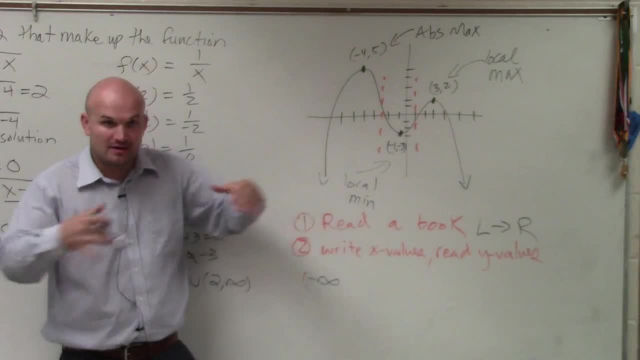 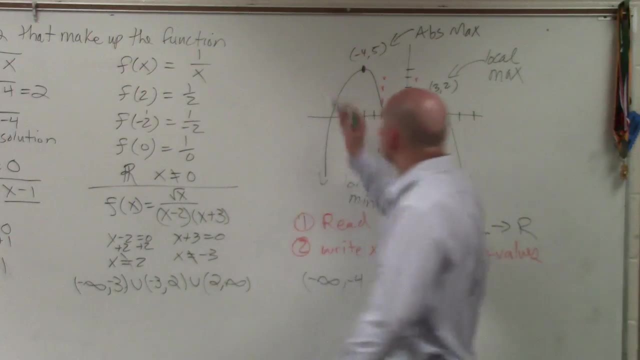 Increasing Right. The y values were increasing right, From negative infinity, from the x value- negative infinity- to negative 4, the graph was increasing. So you'd write negative 4.. Now is negative 4 a part of this graph? Yes, So it's a parenthesis. It's included, right. 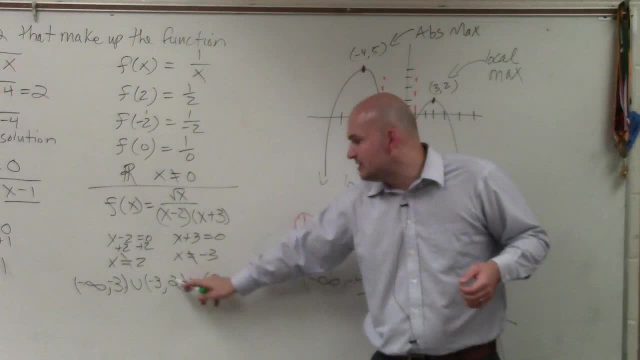 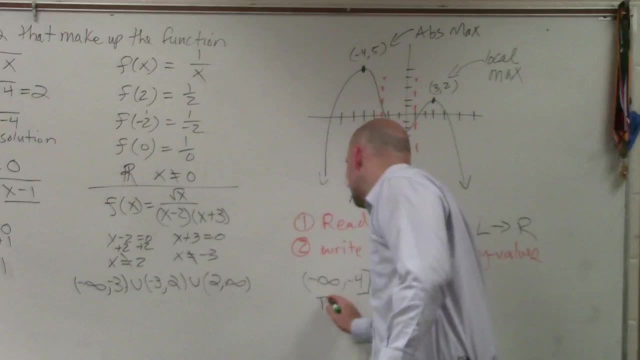 I didn't do that for domain and range over here, Because 2 and negative 3 aren't included. Those are undefined, So we use parenthesis Then, so it's increasing. This is not domain and range, though, so I'm not going to union them, I'm just going to put a comma. 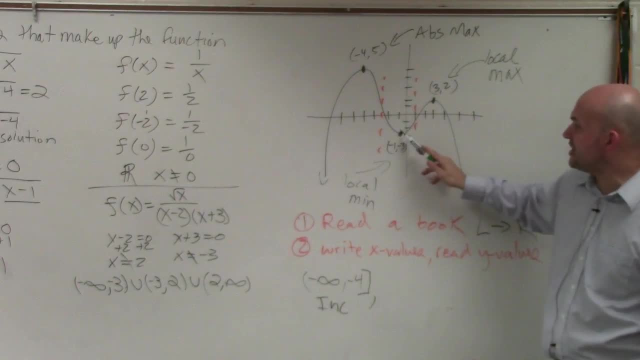 Then from the x value negative 4, to the x value negative 1,. the y values are doing what? Decreasing? So you'd write from negative 1,- oops, I'm sorry- from negative 4 to negative 1, the graph is decreasing. 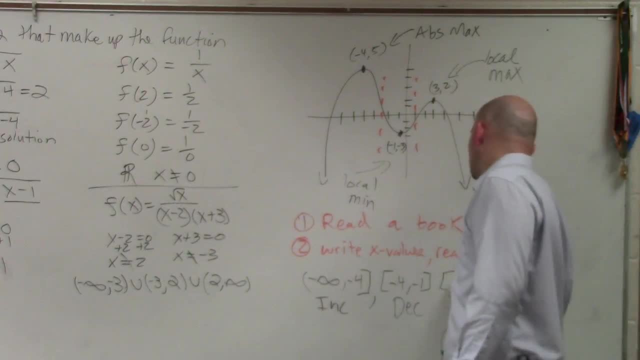 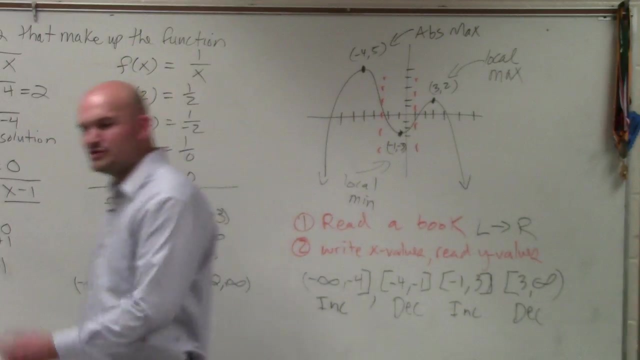 From negative 1 to positive 3, it's increasing, And from 3 to infinity it's decreasing. Does that kind of make sense? Just understand what students get trouble with is they want to use the y values instead of the x values. Read the graph from left to right.